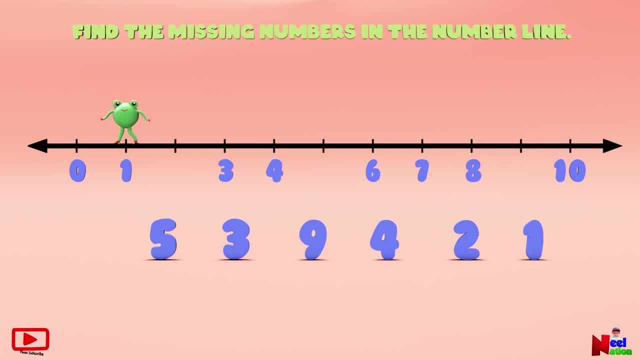 Let's begin with the number 0. And then number 1.. Uh oh, the number after 1 is missing: 1. What comes after number 1?? Number 2.. Yes, you are right. Then number 3.. Then 4.. 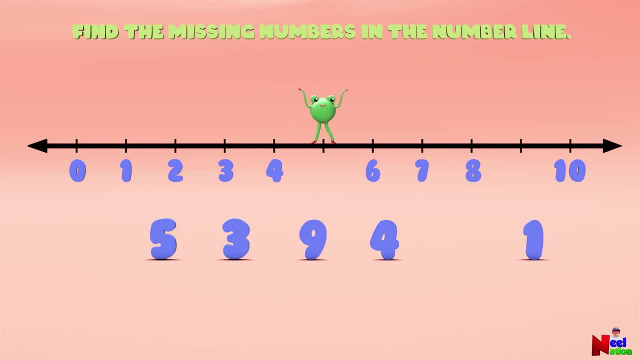 Uh-oh, the number after 4 is missing. What comes after number 4? 5.. Yes, you got it. Number 5. Then comes 6.. 7. Then 8.. The number after 8 is missing. 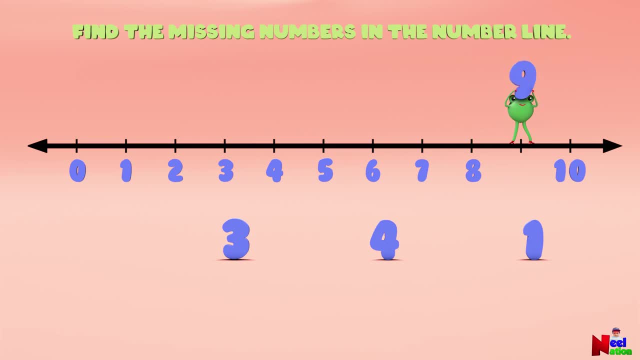 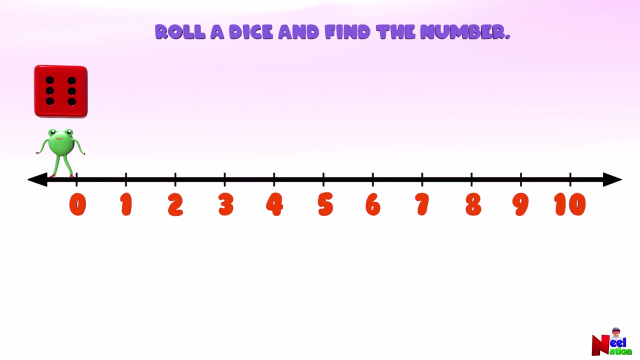 What comes after number 8? Number 9.. Number 9. You are right. And then, finally, is number 10.. You did it again. Great job, I did it. Let's play a game: Roll a dice and find the number. 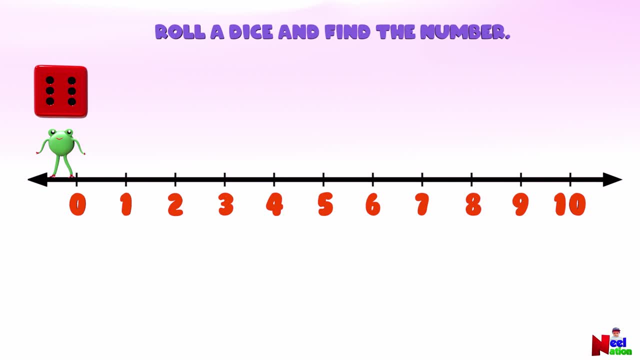 Mr Lutu will play along. Hey, Mr Lutu, Can you please roll the dice? The dice shows the number 2. 2. You are right. Can you locate number 2 on the number line? There you go. 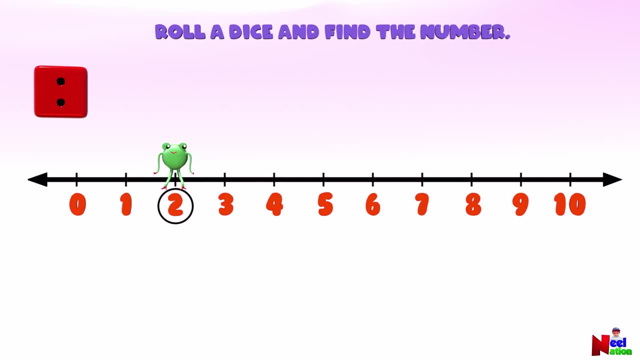 Now can you find the number that comes after number 2? To know that you need to take one jump forward To the right, Mr Lutu has landed on the number 3.. The number after 2 is 3.. 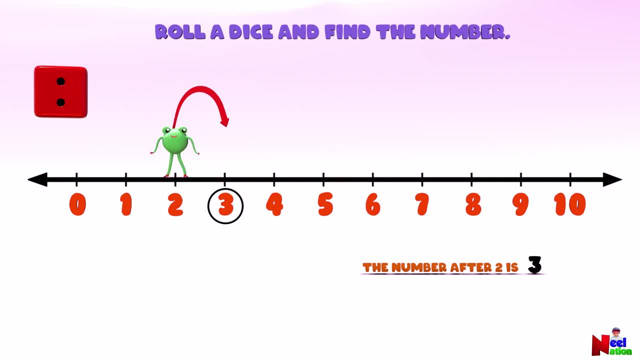 Number 3.. Mr Lutu is back on number 2.. Now can you find the number that comes before number 2? To know that you need to take one jump backwards to the left. Mr Lutu has landed on the number 1.. 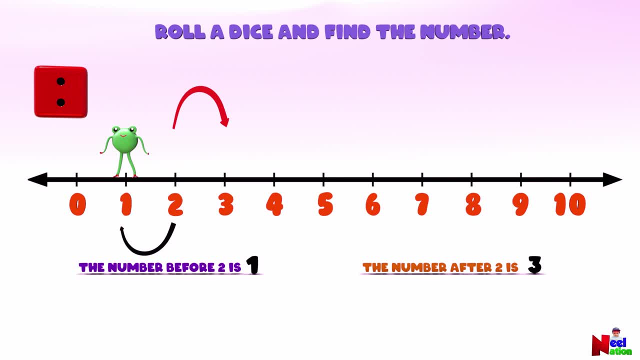 The number before 2 is 1.. One more time. The dice shows the number 5.. 5.. You are right. Can you locate number 5 on the number line 2.. There you go. Now can you find the number that comes after number 5?? 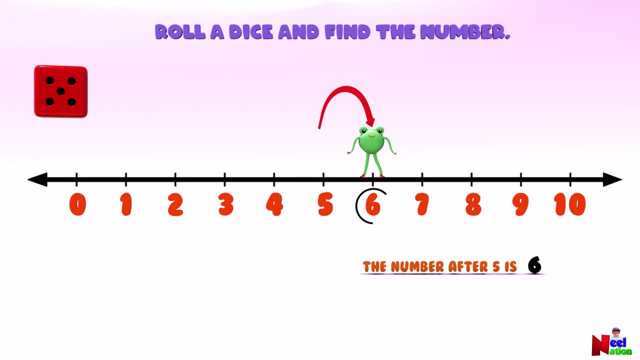 6. The number after 5 is 6.. Mr Lutu is back on number 5.. Now can you find the number that comes before number 5? 4.. You are right. You are right. Now let's look at more and less in a number line. 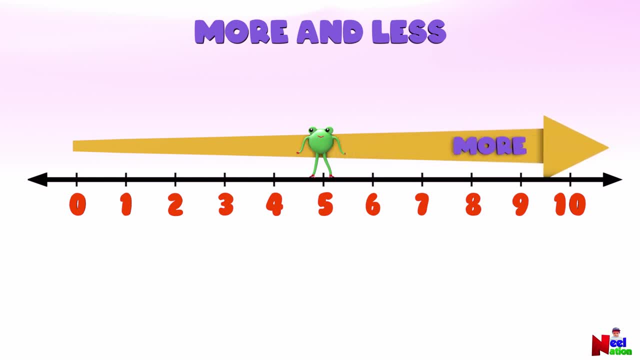 As we have already seen, when Mr Lutu jumps to the right, the numbers keep getting bigger, or it is more, More. And as Mr Lutu jumps to the left, the numbers keep getting smaller or it is less. 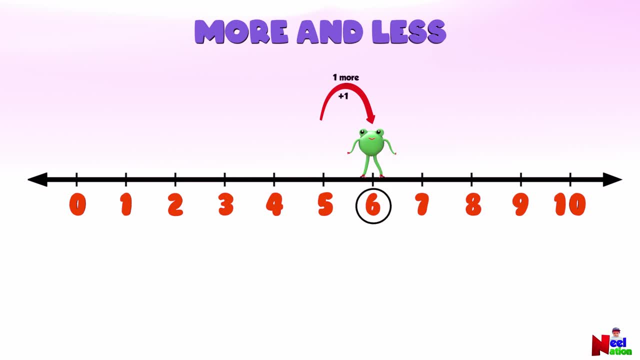 Less. So when Mr Lutu jumps one point to the right, it is one more, That is one more, One more again. Now look closely. Mr Lutu is going to take a giant leap: two points to the right, and that is two more. 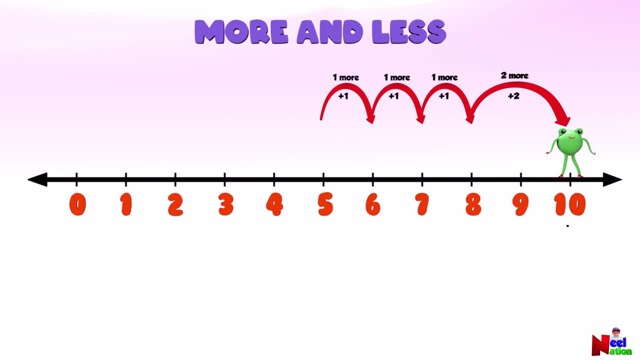 Two more. So when Mr Lutu jumps one point to the left, it is one less, One less. That is one less, One less, again One less. Now look closely, Mr Lutu is going to take a giant leap: two points to the left and that is two less. 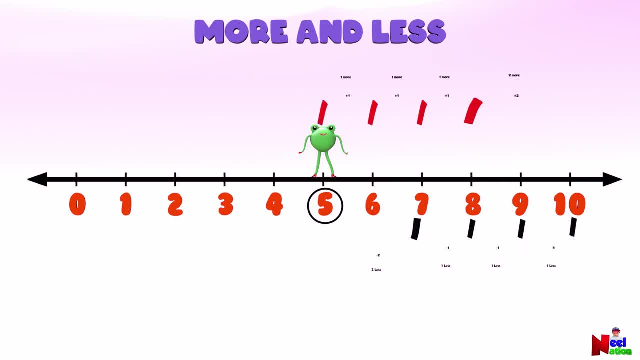 Two less. Now let's do a fun activity. Let's make Mr Lutu do a couple of jumps. Mr Lutu is now on number 5.. Hey, Mr Lutu, can you find the number one less than number 5?? 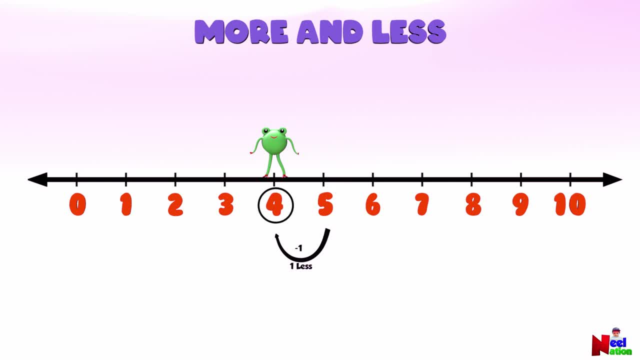 Number 4.. Number 4.. You got it Okay, Mr Lutu. Can you find the number two less than number 4?? Number 2. Two, Perfect. Okay, Mr Lutu. What is one more than number 2?? 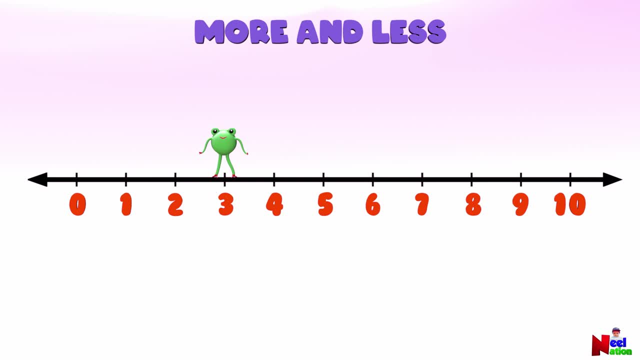 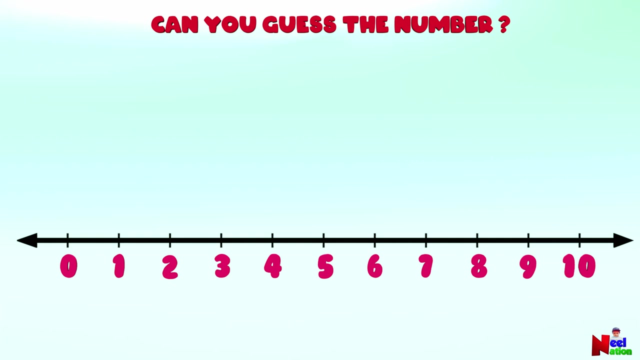 Number 3. Three, You got it Okay. here comes the tricky one. What is three more than number 3?? Number 6. Number 6. Awesome, Good job, I have some clues for you. Can you guess the number? 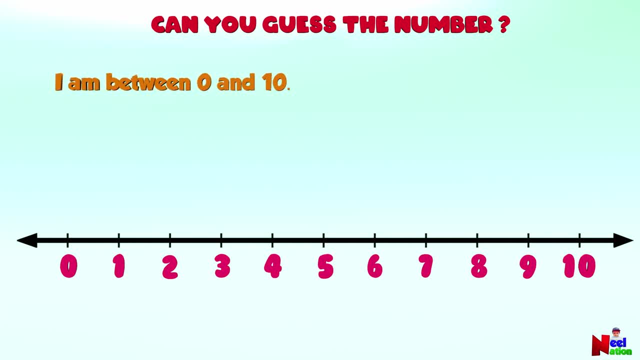 Yes, I can do it. I am between 0 and 10.. I am more than 5.. I am the number before 8.. What am I? Can you guess the number? Let's look at the clues one more time. 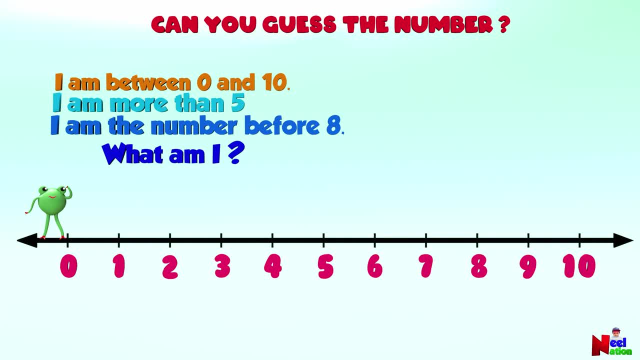 I am between 0 and 10.. I am more than 5.. I am the number before 8.. Number 7.. Yes, that is number 7.. You got it Okay. let's get to the next guess. I am between 0 and 10.. 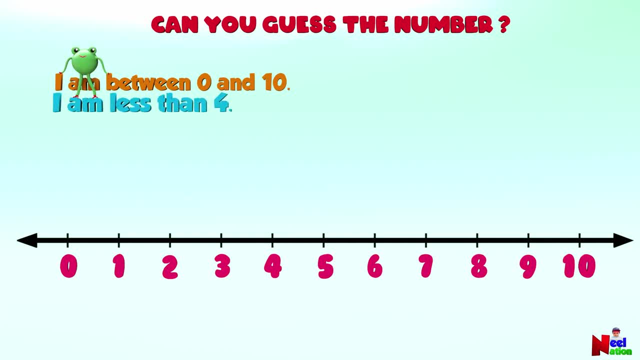 I am less than 4.. I am the number after 1.. What am I? Can you guess the number? Let's look at the clues one more time. I am between 0 and 10.. I am less than 4.. 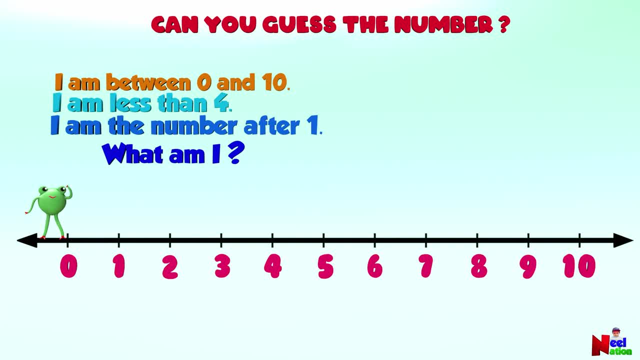 I am the number after 1.. What am I? Number 2. Yes, the number is 2.. You are awesome. Okay, let's learn one more time. Number 7.. Number 7.. Number 8.. Number 9.. 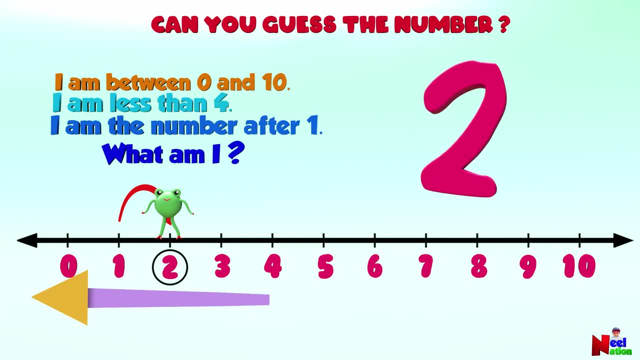 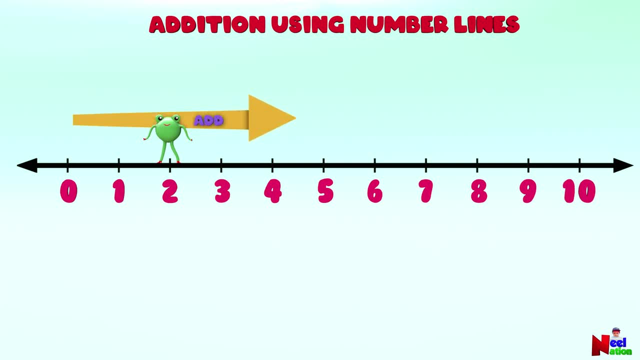 Number 10.. Number 11.. Number 12.. Number 13.. Number 14.. Number 15.. Number 16.. Number 17.. Number 18.. Number 19.. Number 20.. Number 21.. Number 22.. 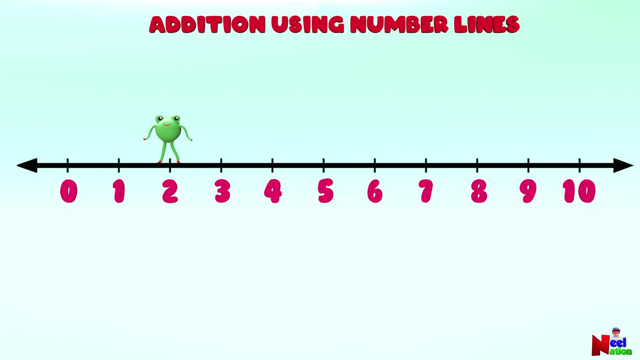 Number 23.. Number 24.. Number 25.. Number 26.. Number 27.. Number 28.. Number 29.. Number 30.. Number 31.. Number 32.. Number 33.. Number 34.. Number 35.. 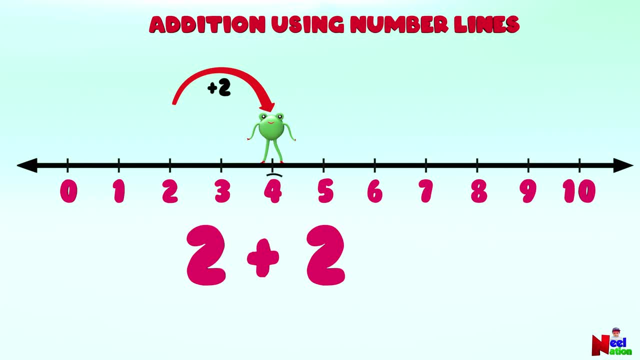 Number 36.. Number 37.. Number 38.. Number 39.. Number 40.. Number 41.. Number 42.. Number 43.. Number 44. Number 45.. get four. two plus two is four. two plus two equals four. one more time, mr lutu is at the number five.